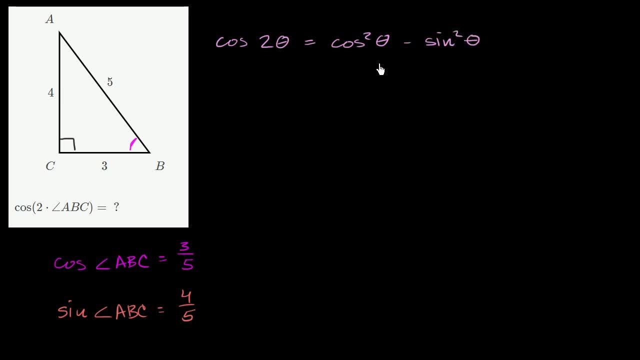 squared minus sine of that angle squared, And we've proved this in other videos. But this becomes very helpful for us here, Because now we know that the cosine of angle ABC is going to be equal to the cosine of 2 times the angle ABC. 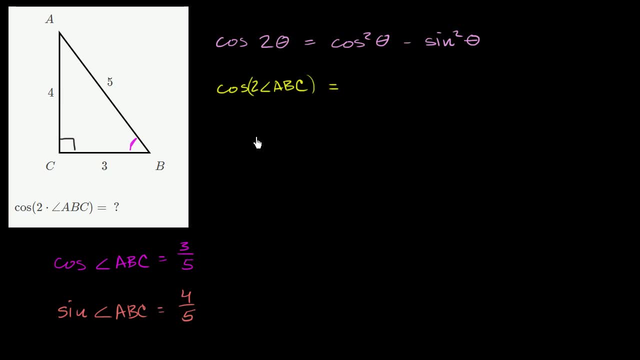 That's what we care about. 2 times the angle ABC, It's going to be equal to the cosine of angle ABC squared minus sine of the angle ABC squared. And we know what these things are. This thing right over here is just going to be equal to 3 fifths squared. 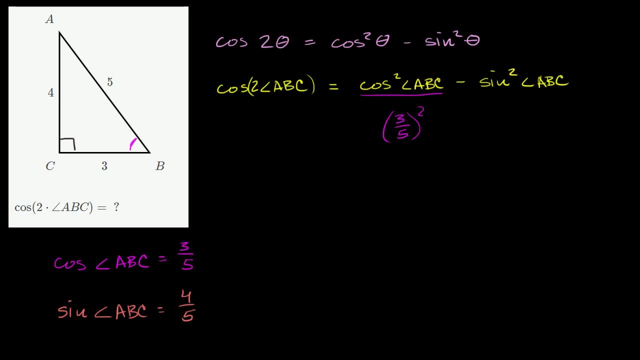 Cosine of angle ABC is 3 fifths, so we're going to square it And this right over here is going to be equal to 3 fifths And this right over here is just 4 fifths squared, So it's minus 4 fifths squared. 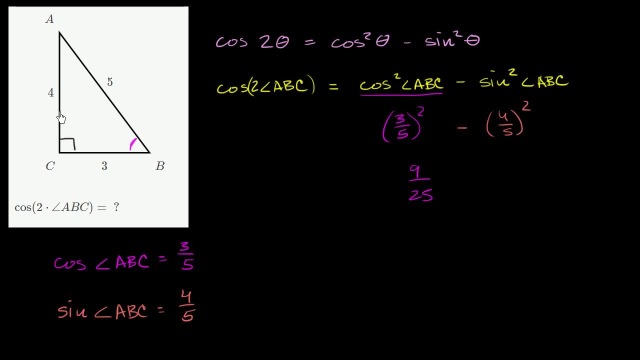 And so this simplifies to 9 over 25 minus 16 over 25, which is equal to 7 over 25.. So this thing right over here is equal to 7.. Sorry, it's negative. Got to be careful there. 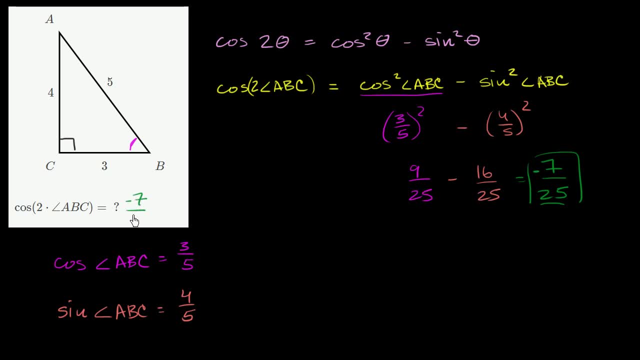 16 is larger than 9.. Negative 7 over 25.. Now one thing that might jump at you is: why did I get a negative value here when I doubled the angle here? Because the cosine was clearly a positive number. And there you just have to think of the unit. 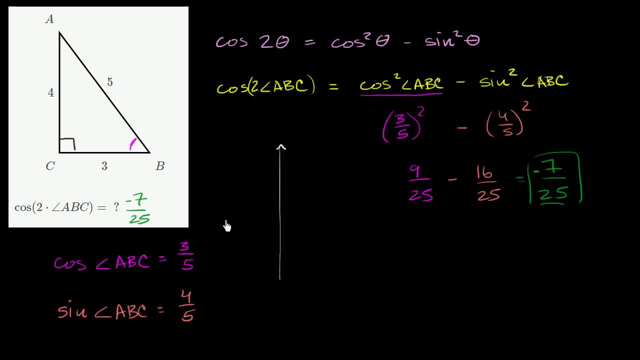 circle which we already know is an extension. The unit circle definition of trig functions was an extension of the SOHCAHTOA definition x-axis, y-axis. Let me draw a unit circle here, My best attempt. So that's our unit circle. 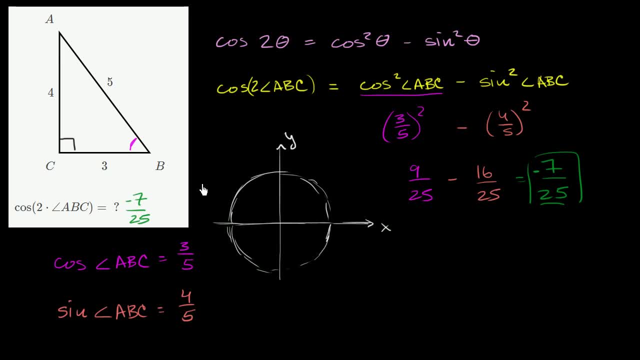 So this angle right over here, Right over here, looks like something like this. So it looks like something like this, And so you see its x-coordinate, which is the cosine of that angle, looks positive. But then if you were to double this angle,